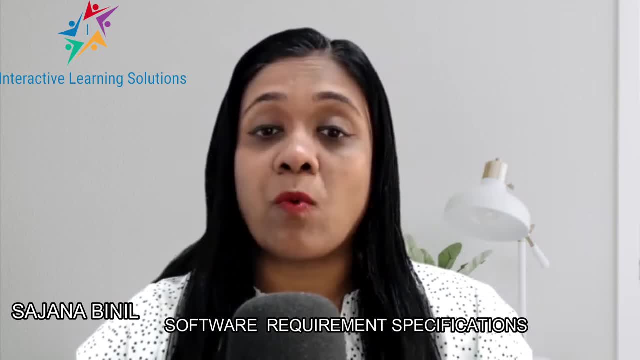 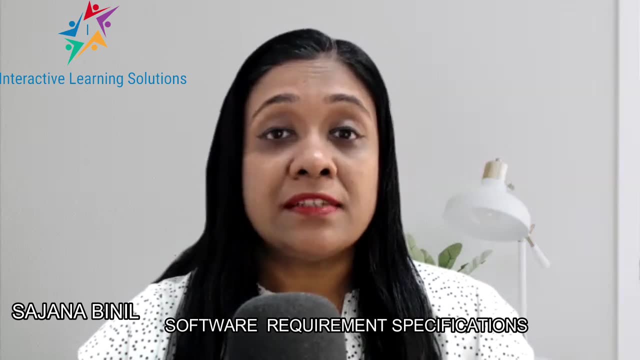 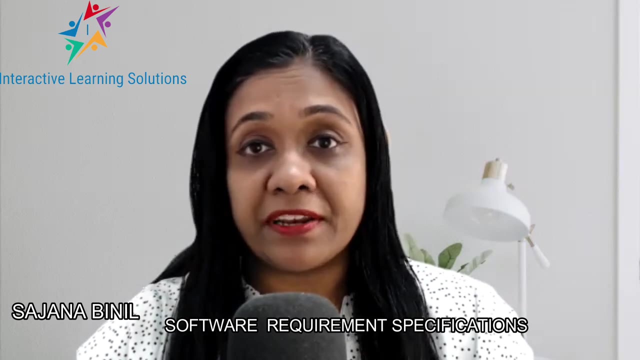 What it contains. It contains detailed functional requirements and non-functional requirements, along with use cases And who uses this document? This document is used by project managers, SMEs, technical team and the implementation leads. When is this document prepared? This document is prepared in the planning phase. 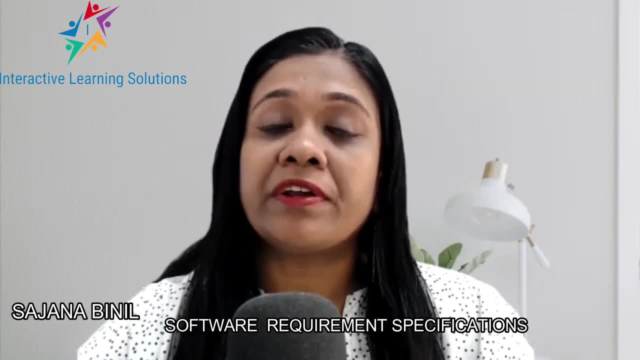 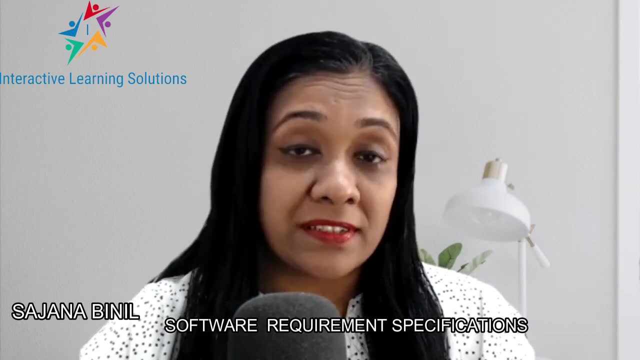 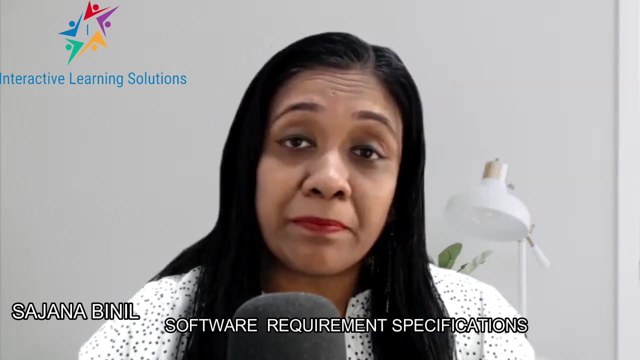 And this document answers the question: what requirements must be fulfilled and what is included in this document? Well, this document primarily answers the question: what requirements must be fulfilled in order to satisfy the business needs. Now let's take a look at an example of a system requirement. 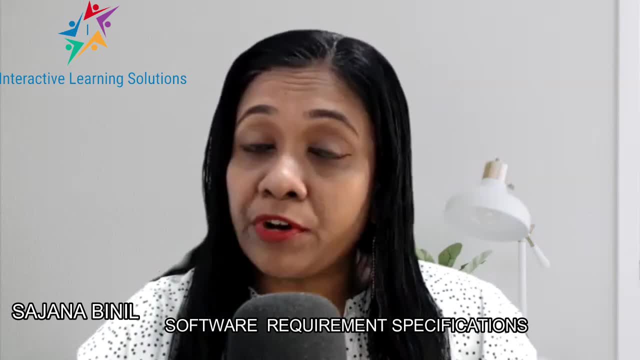 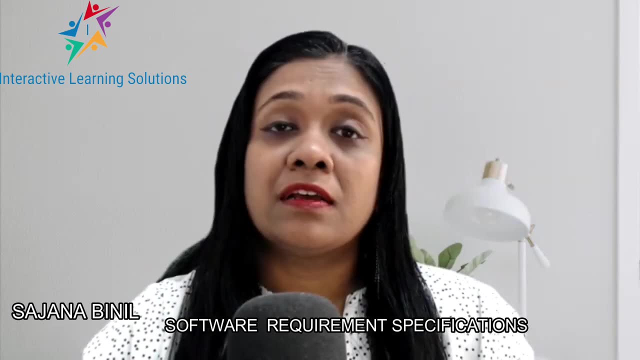 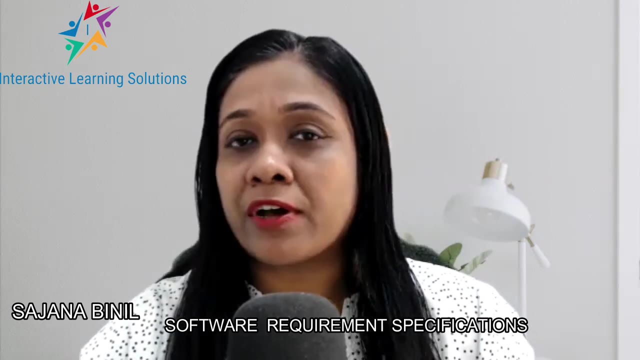 The proposed software should contain the following modules: login, registration, search, employee and reporting administration- So net-net. in a system requirement document we indicate what kind of functionality should be included in the product that we are building for our customer. Let's take a look at the third document: Functional Requirement Document. 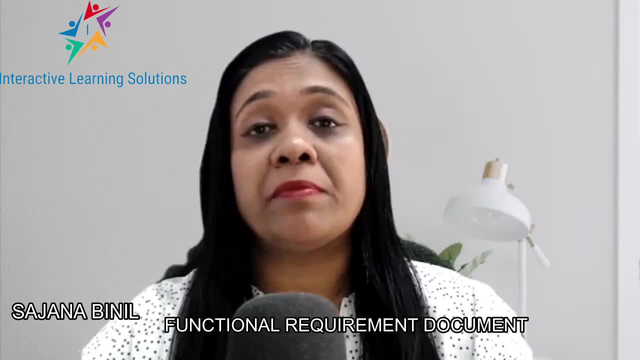 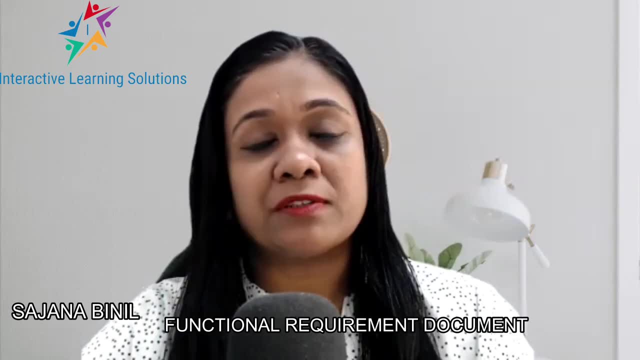 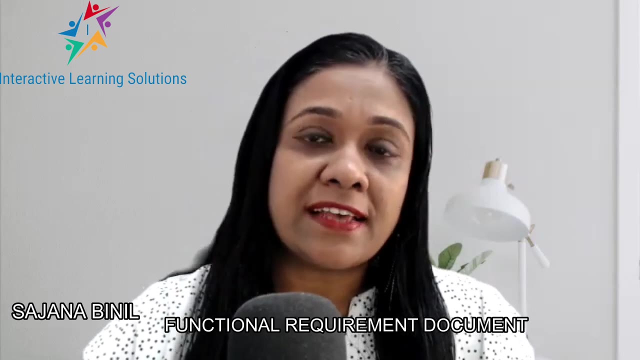 This document is also called as Functional Specifications Document, Product Specifications Document and Functional Specs. Who prepares this document? This document is prepared by the business analyst or the system analyst. Now, what is the difference between an SRS and FRD is something that you need to understand. 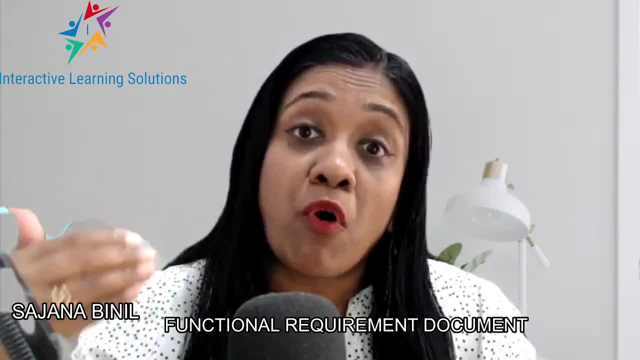 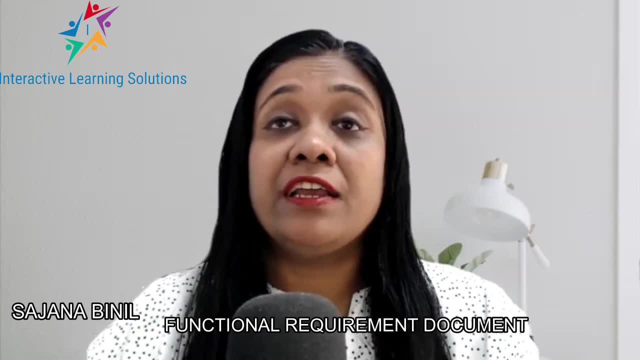 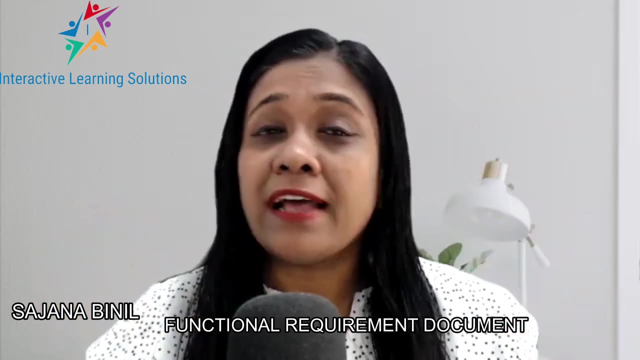 While the SRS tells you what kind of functionality or what kind of modules should be included in your system, the FRS will give you much more granular information. It will tell you what kind of data should be shown in each and every screen and what overall and the overall behavior of the system. 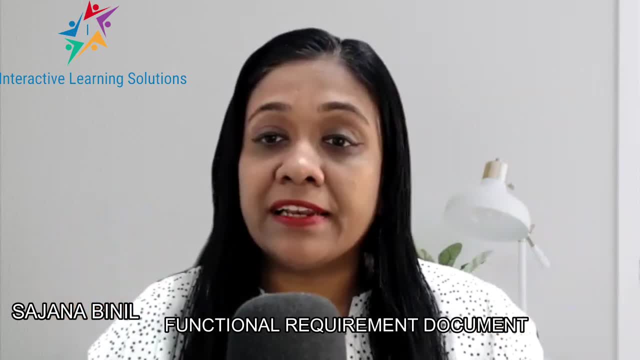 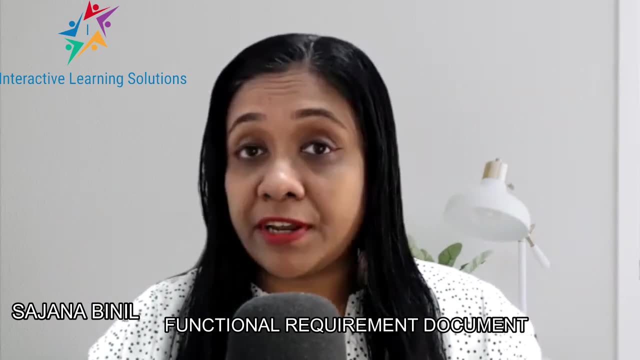 Who uses this document? This document is used by the technical team, The technical leads, the development teams, the testing team and also your customer. When is the FRD prepared? Well, an FRD is prepared in the planning phase, And what is the question it answers? 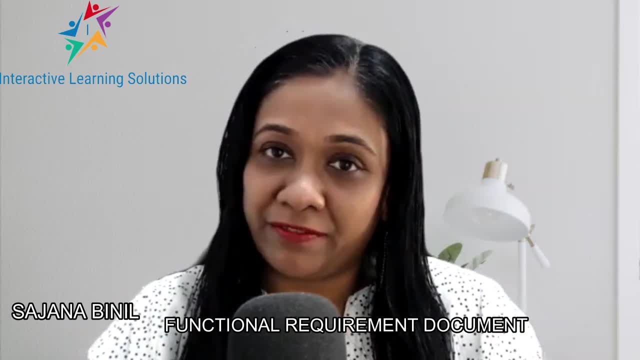 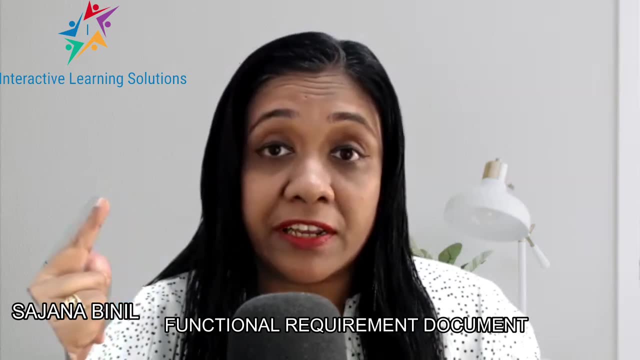 It answers the question how exactly the system is going to behave. Please note: when I'm saying how the system should behave, it doesn't mean that the FRD will include implementation details like code snippets, database details. It will only include details about the behavior.